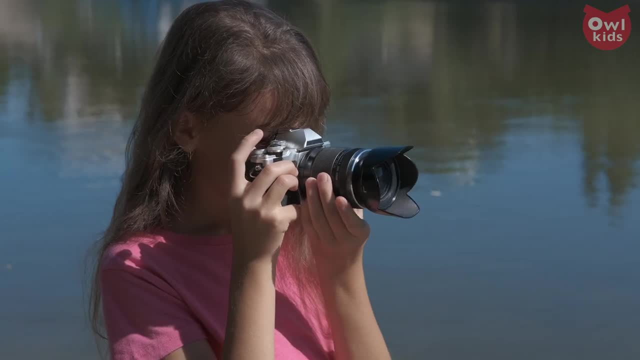 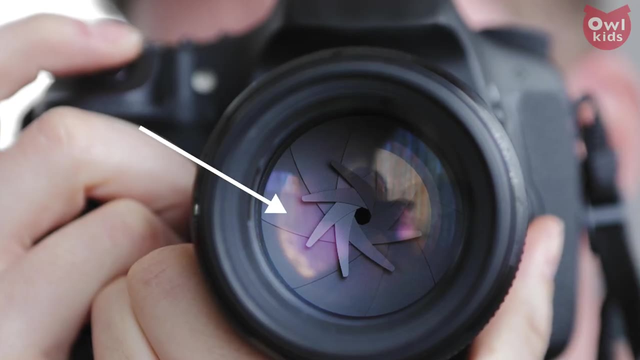 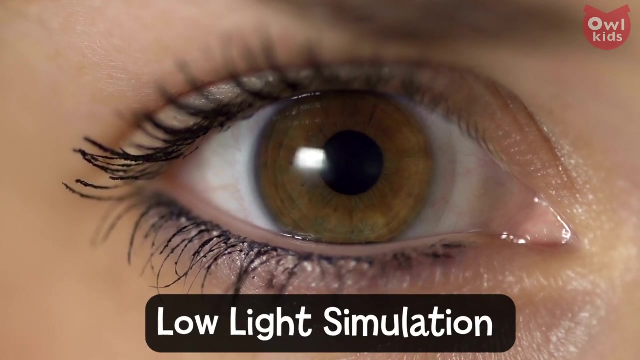 at the front that can expand or contract to control how much of that light gets inside. On the eye it is called the iris. On a camera it is called the diaphragm. Here's how the iris works In low light. it will expand to let in as much light as possible. 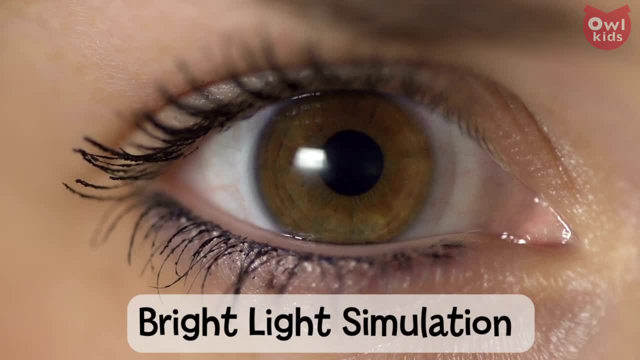 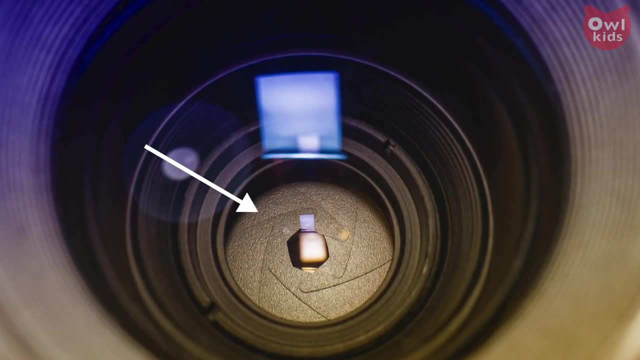 This helps us to see, But in bright light it contracts so that our eye does not get overwhelmed. The camera's diaphragm works in the same way. At the center of the diaphragm is an opening called the aperture. By changing the aperture's setting, we can get well-lit images. 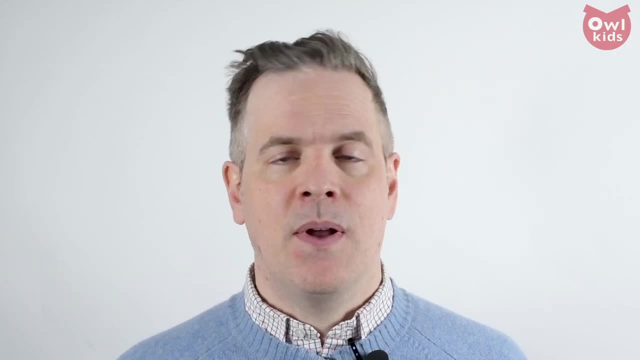 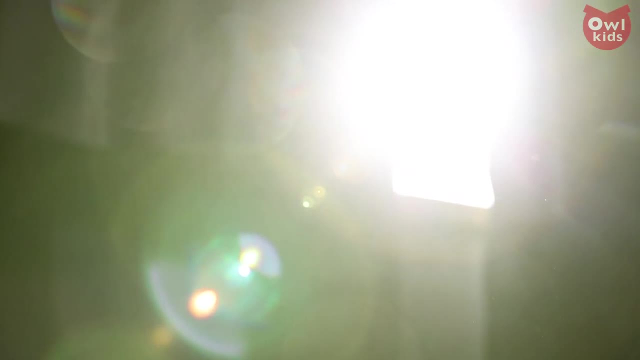 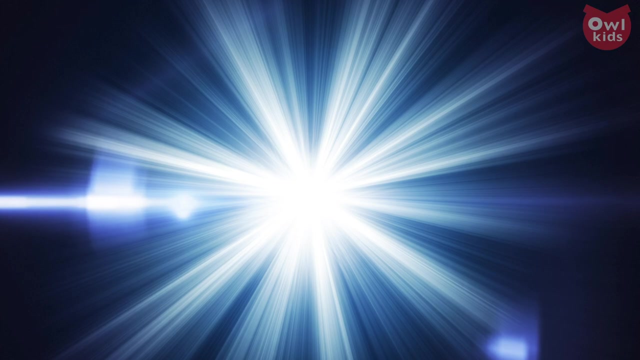 in a variety of situations. But there's a lot more to a camera than simply letting light inside it. Let's talk about light for a second, especially how it moves. Light is electromagnetic radiation and it travels in waves, Waves that move in all directions at once. A light source. 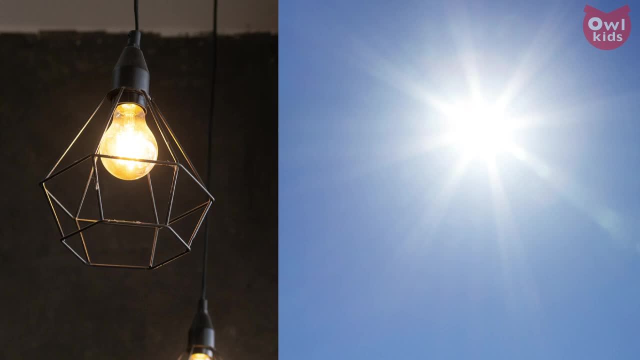 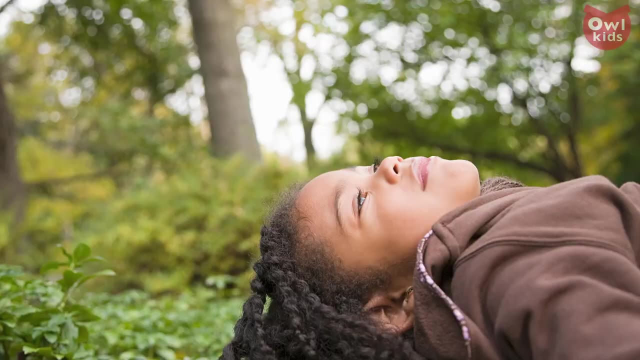 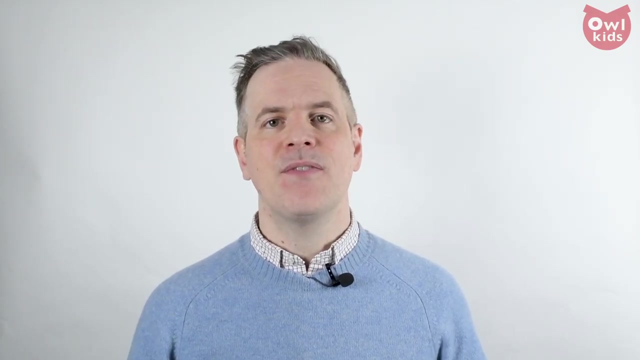 such as a light bulb or the sun, creates its own light waves, But most other things, including us humans, only reflect light. As light waves hit us, they bounce back off, revealing us to the world. However, that reflected light bounces off of us in all. 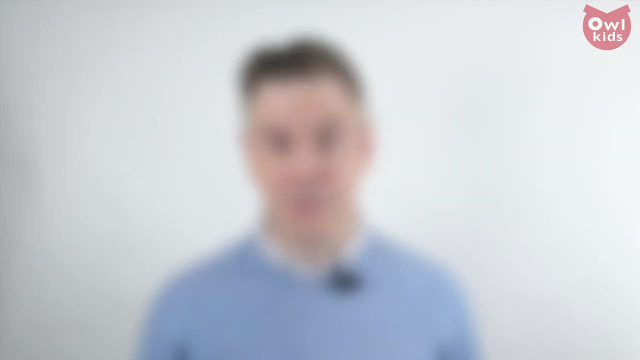 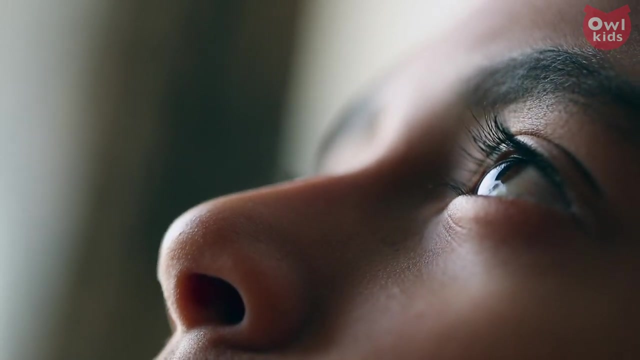 directions at once, making us appear as a blur. Thankfully, the human eye is able to capture and focus that light into what is known as a real image. To successfully take a picture, a camera needs to create its own real image, And to do that, 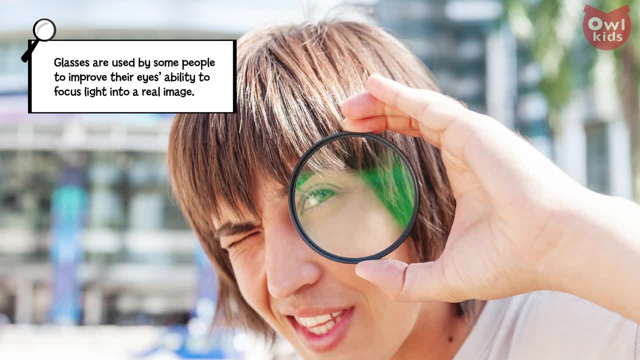 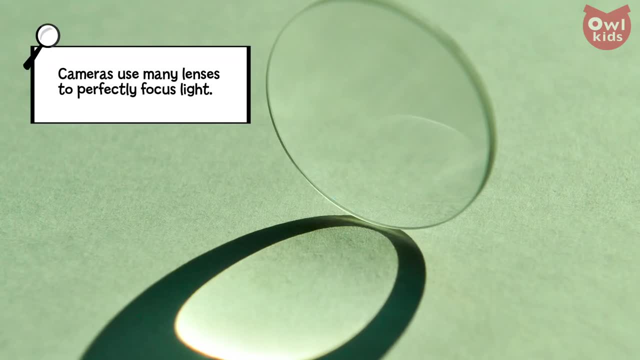 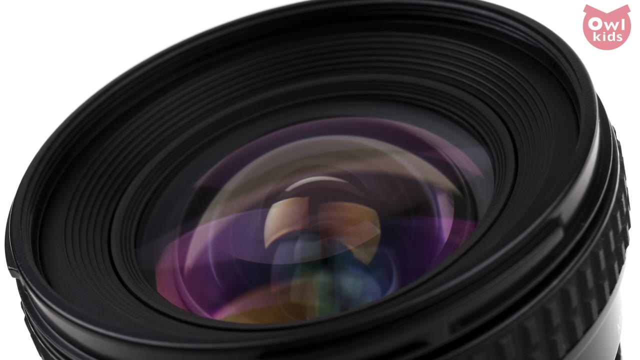 it uses lenses In the most basic sense. a lens is a piece of curved glass or clear plastic. As light passes through the lens, this curve causes the direction of the light to bend. A camera uses a convex lens. This is where the lens bends outward like a gentle hill. 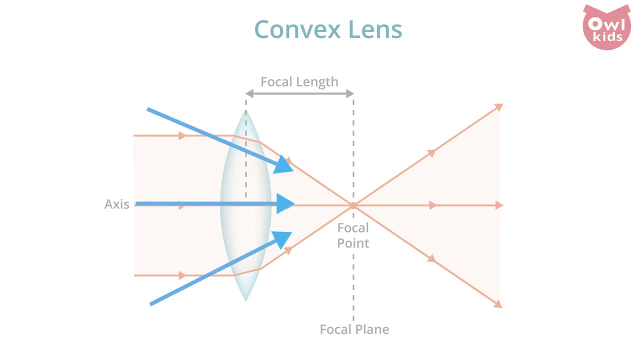 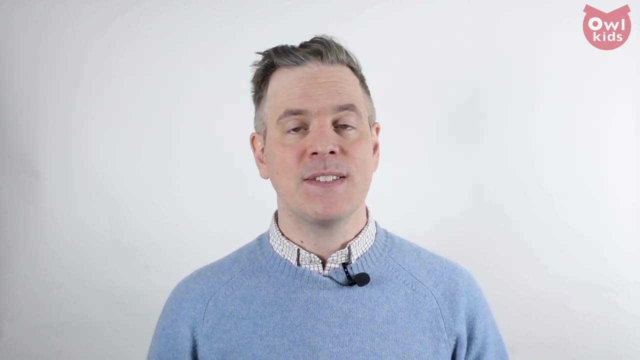 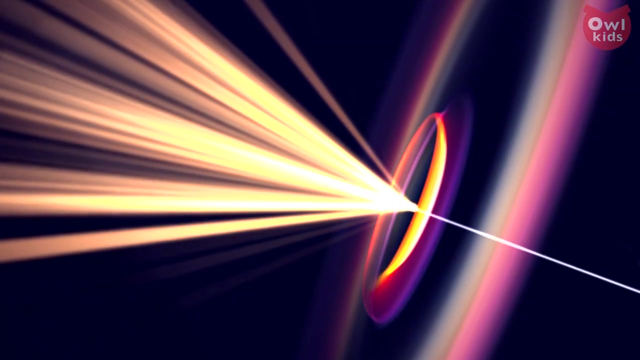 When light passes through a convex lens, the rays converge or meet at a central point. Now all those waves of light that were flying off in every direction have been focused together. After converging, the rays will begin to spread apart again. Fortunately, we want this to happen As the rays begin to spread apart. 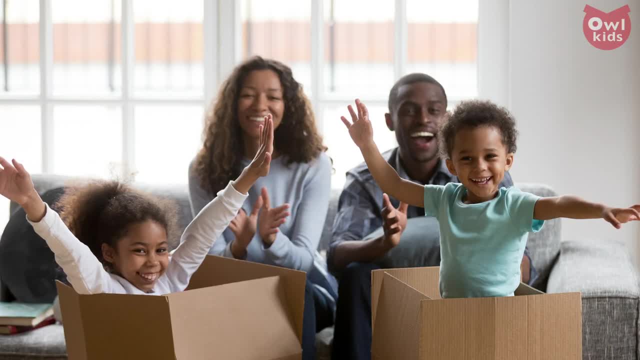 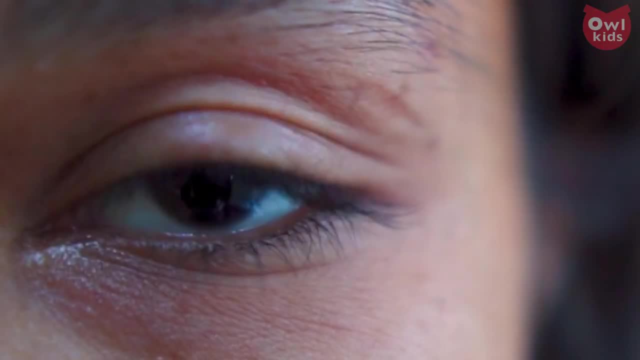 they open up to create our real image. The only difference is because the beams have crisscrossed. that image is actually flipped upside down. Incidentally, the same thing happens inside our eye, but our brain doesn't, So instead we need to make sure it's actually front-facing, But in reality,